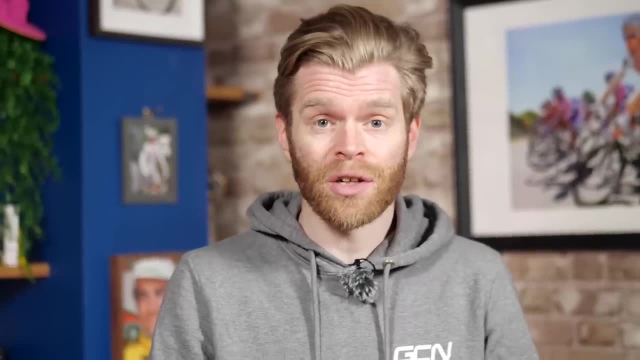 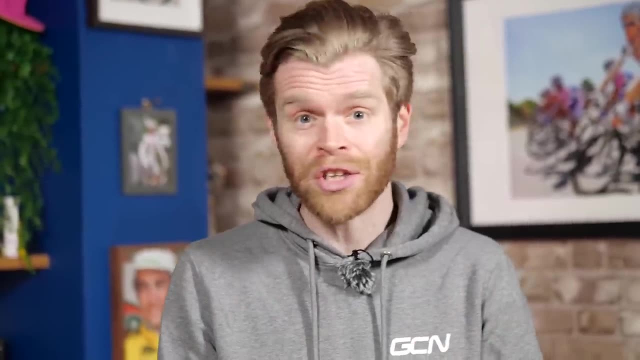 to comment and subscribe if this is something you wanted to see. Turned out a lot of you did, and so here it is. We aim to make the videos that you want. If you appreciate this kind of stuff and you haven't yet subscribed, please do, because it really helps. 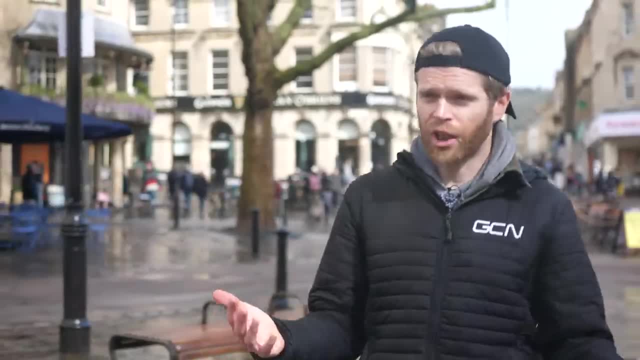 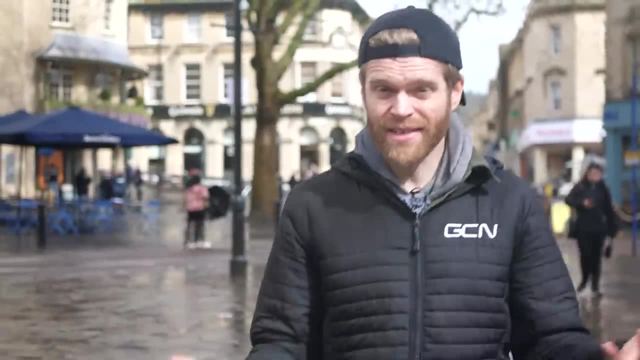 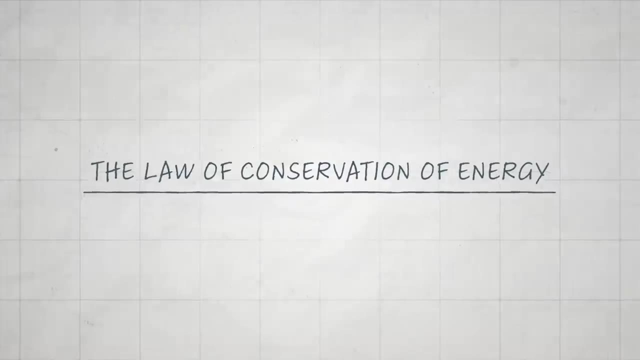 Calorie counting doesn't work, or does it? Counting and restricting the number of calories you eat? Regarding Calorie counting: Calorie counting: Total Energy at Time 2 Minus Total Energy at Time 1- sorry Time Sum Calorie count. Calorie counting. 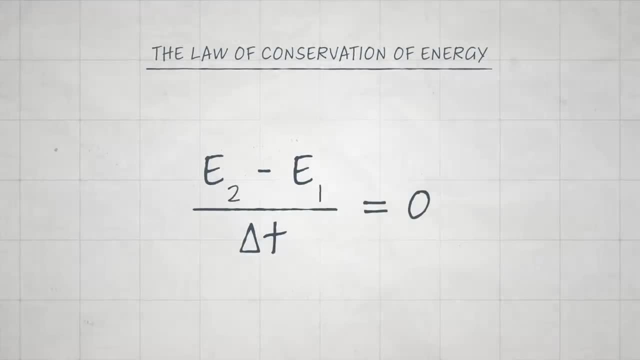 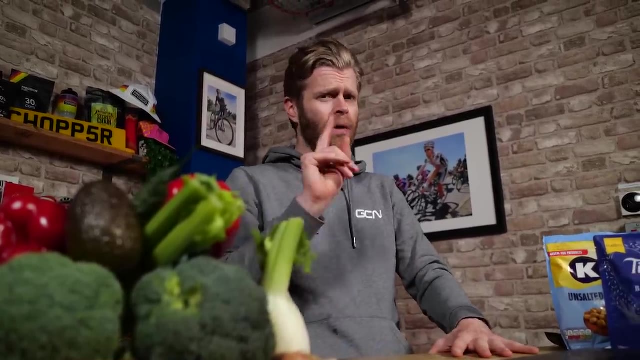 Calorie: debit, gym charge system study video: Calorie: counting the two equals zero. So if you burn more than you take in, you will lose weight. Now, this is true. It's Newtonian physics. The universe wouldn't exist without it. However, there are some problems. 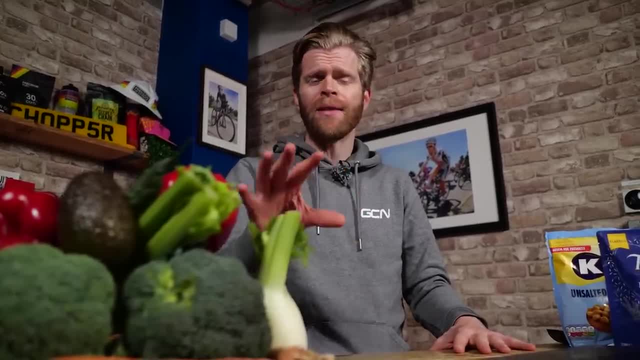 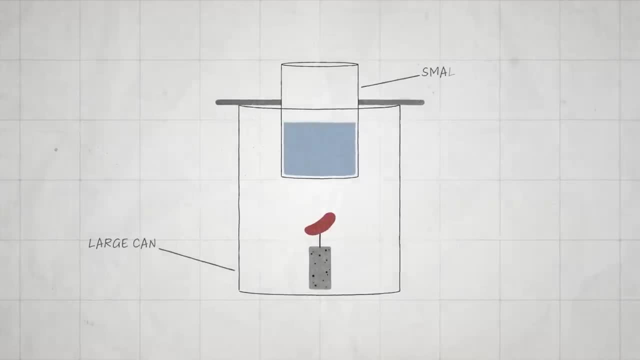 with this gross oversimplification and I will explain that. But first we need a quick refresher on what a calorie actually is. A calorie is defined as the energy required to raise the temperature of one centimeter cubed of water by one degree Celsius by weighing and burning the 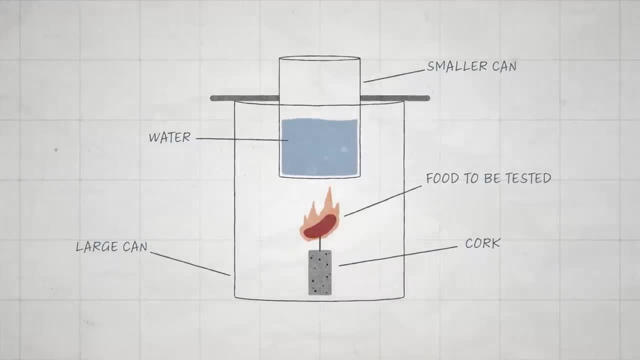 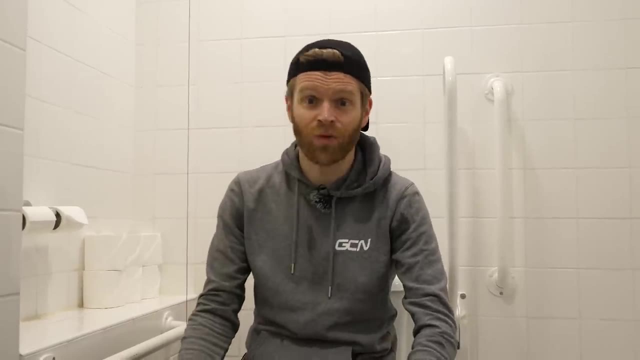 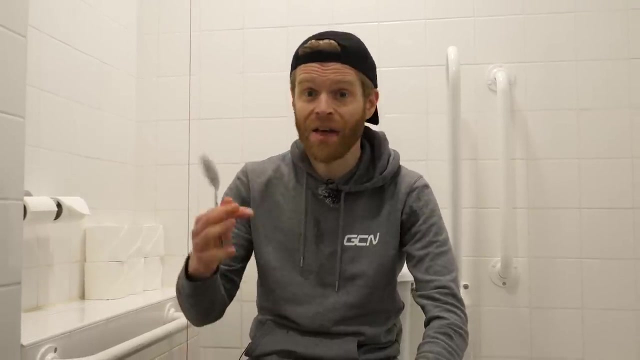 food. These experiments that burnt food were some basic science known as bomb calorimetry, performed in the late 1800s, So as to why calorie counting doesn't work well. reason one: your body is not a bomb calorimeter. When you eat food, it doesn't incinerate it and therefore 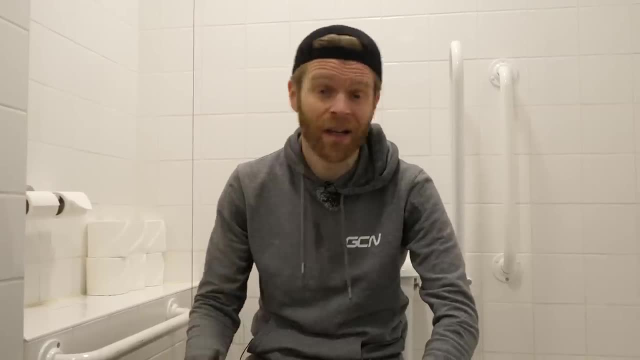 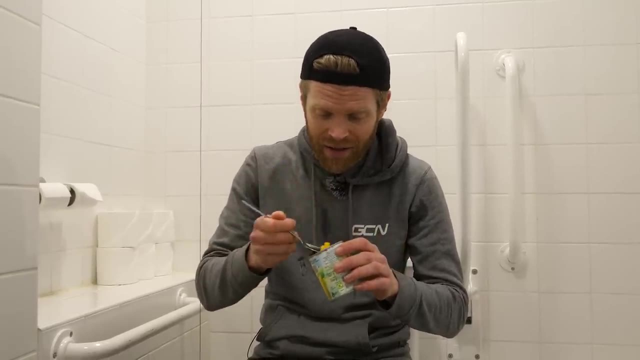 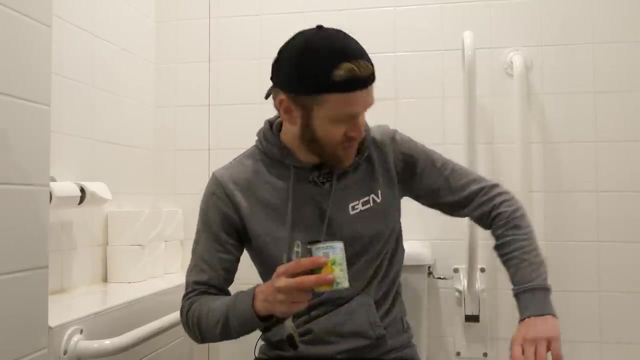 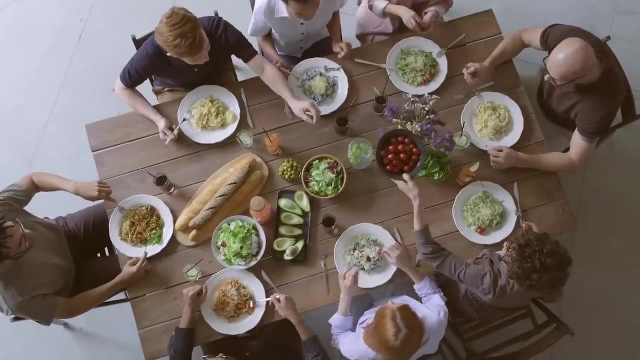 it doesn't necessarily extract all of the nutrients from it. My favorite example of this: sweet corn. Now, well, feel free to join in at home and conduct your own Experiment and then, well, observe the results. And people respond to different foods differently. For example, most Europeans struggle to digest and 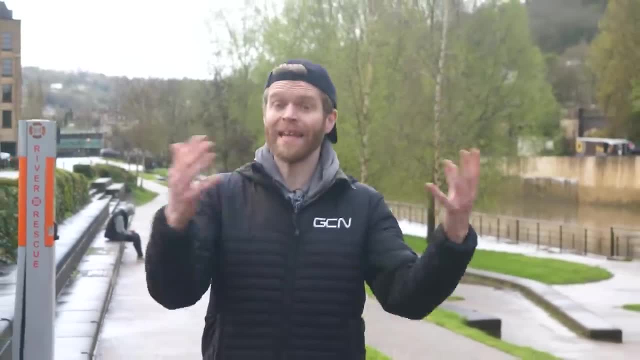 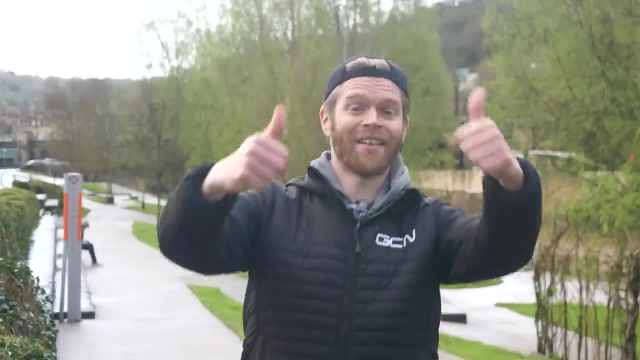 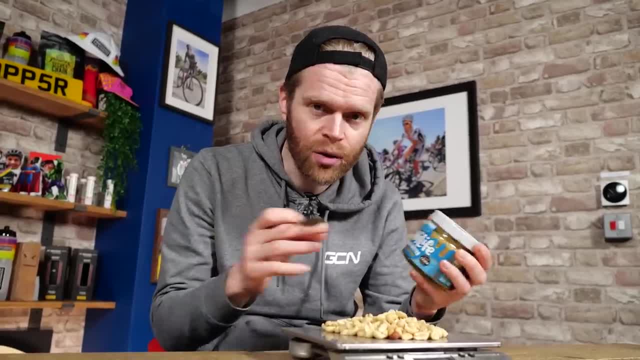 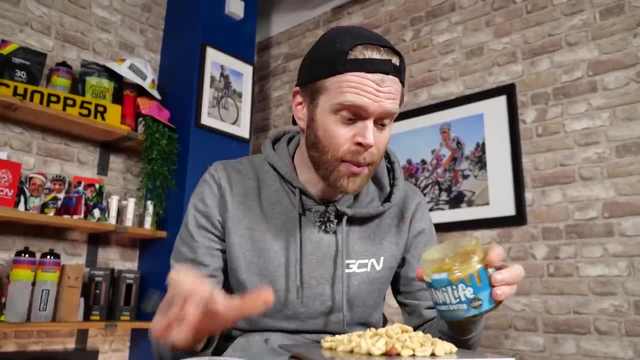 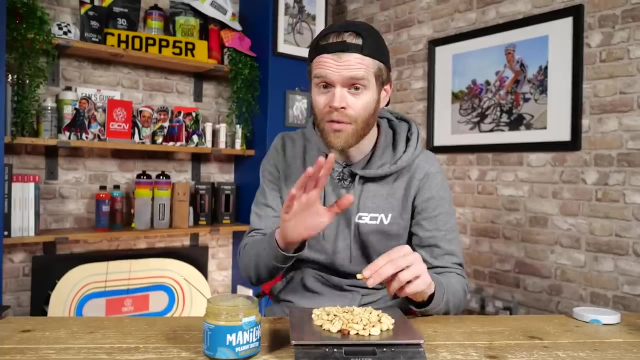 walls contained within the nuts have broken down and then released the oil or fat that's contained within each nut cell, and that's what gives nut butter its yummy and creamy texture, as opposed to it being just a- well, a nutty powder. However, when you eat nuts, your body isn't actually able. 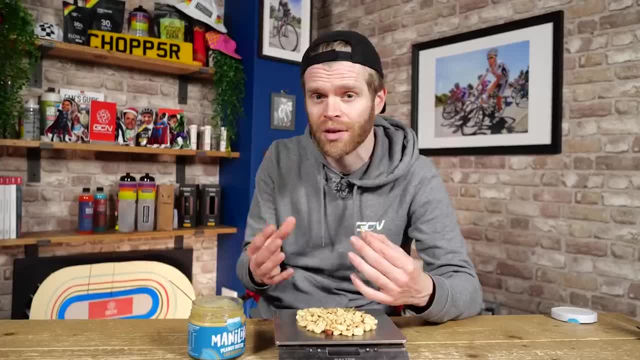 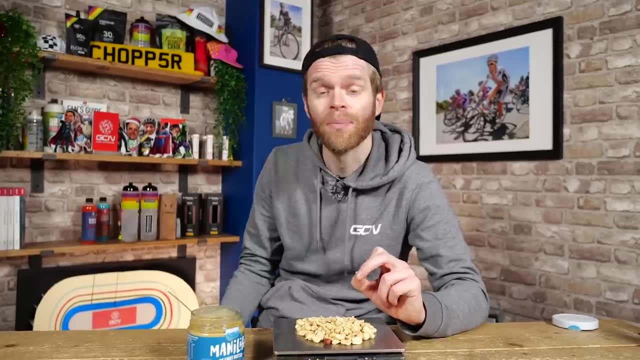 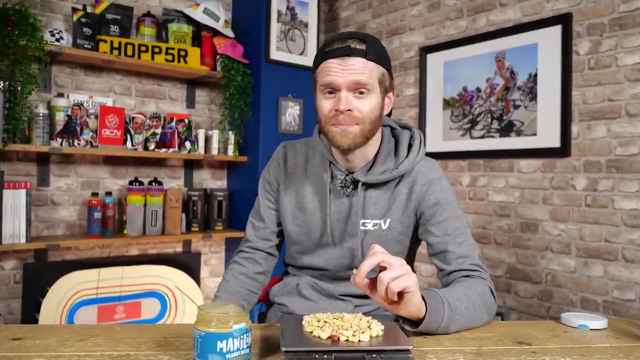 to break down the cell walls of every single nut that you eat and thus release the fat contained within it. We know this because scientists have analyzed the fecal matter from people whom they fed nuts, thus doing this so that you don't have to Thanks science If you were tracking the calories. 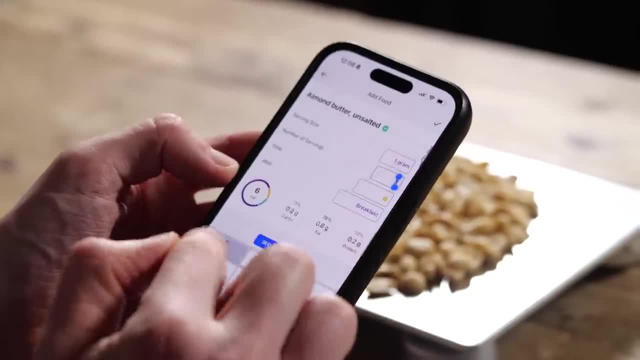 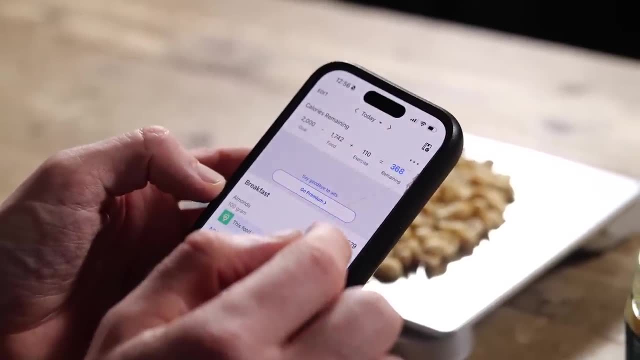 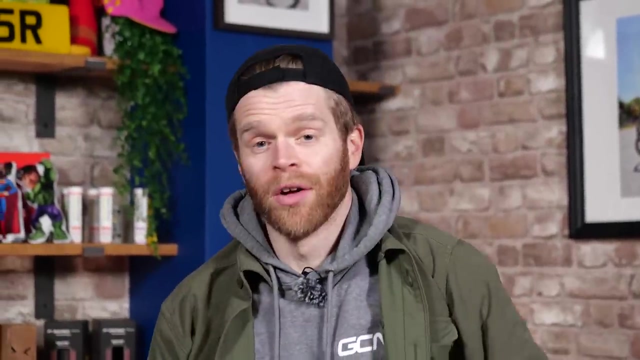 of a hundred grams of nuts. it registers roughly the same if it's a hundred grams of nut butter versus a hundred grams of raw nuts, and this isn't the case. and this is all because of the matrix. No, not that one, the food matrix. It's just a fancy and misleading way of describing the structure of. 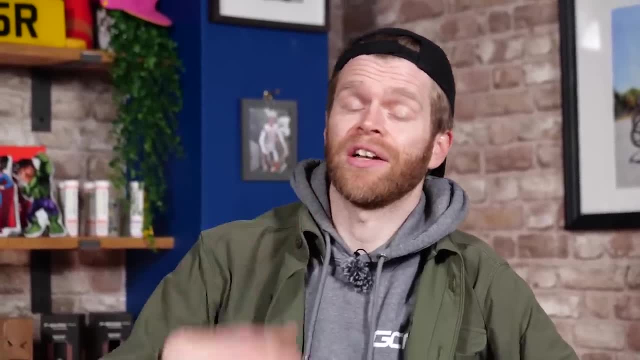 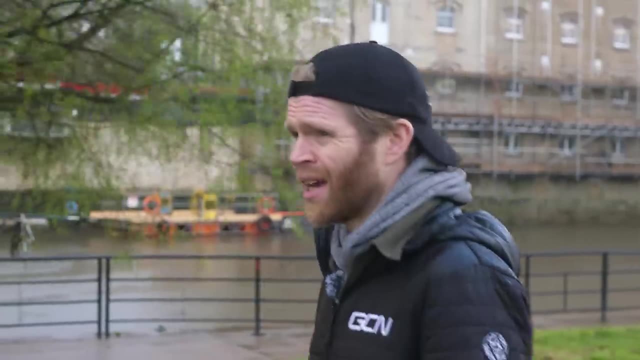 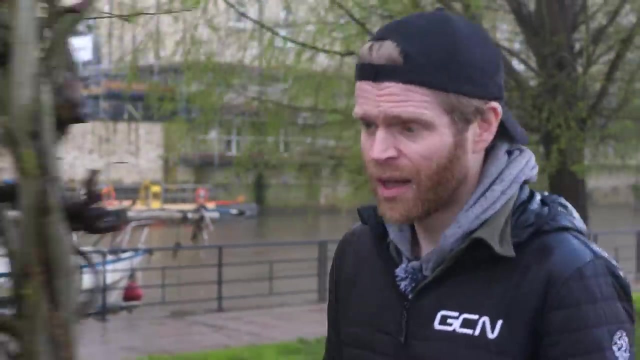 food that well makes it sound far more exciting than what it actually is. Reason two is that, irrespective of how your body individually responds to food, it's very difficult to accurately measure the calories of food that you're just eating before you've even tried to digest them. For example, food labels only have to be 20%. 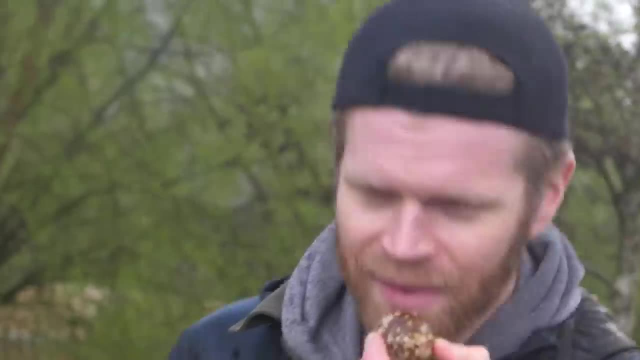 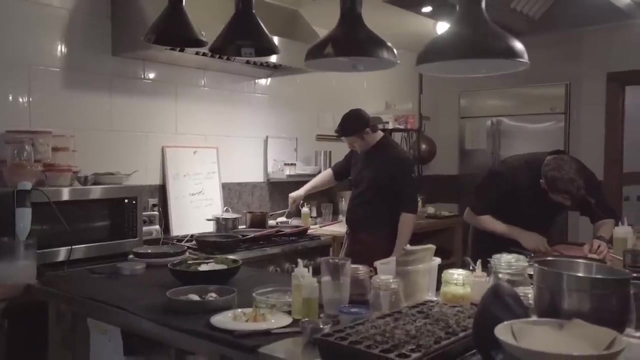 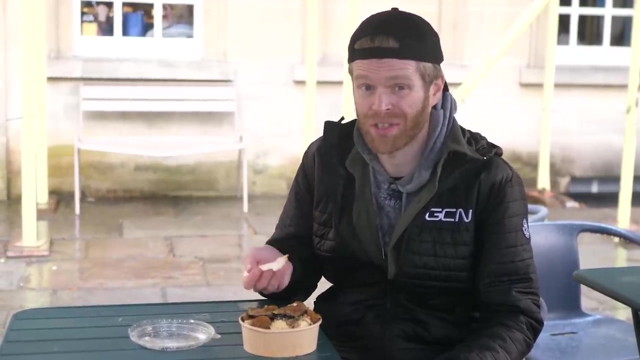 accurate by law, which means that this tasty 100-calorie snack might actually be 120 calories. Homemade meals or dishes prepared in restaurants or cafes often become a complete guessing game. It's impossible to accurately measure and control portion sizes and the actual calories contained. 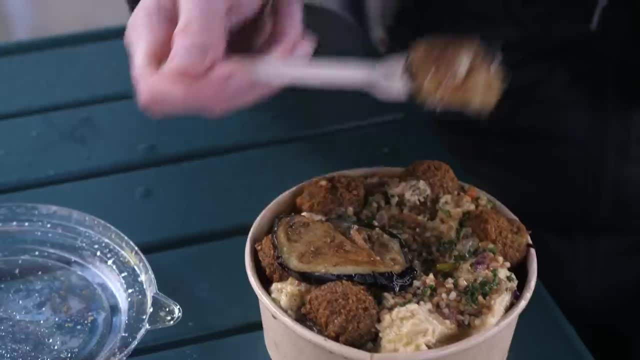 within a meal can vary by over 50%. Even professional dietitians struggle to measure their intakes from things like the amount of food that they're eating, the amount of calories that they're consuming, the amount of calories that they're consuming, the amount of calories that they're. 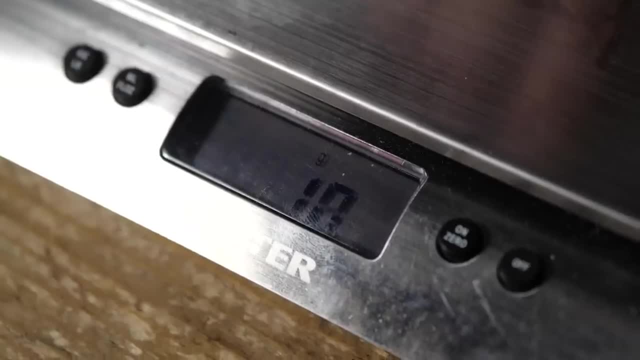 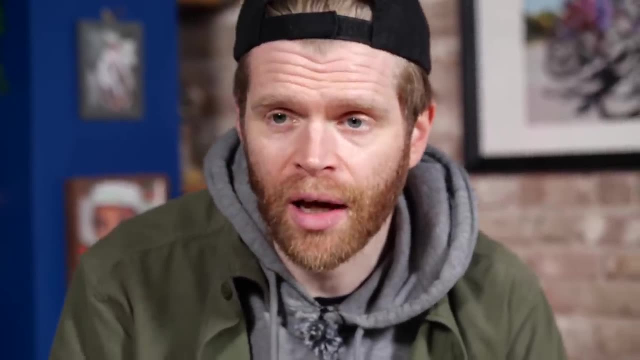 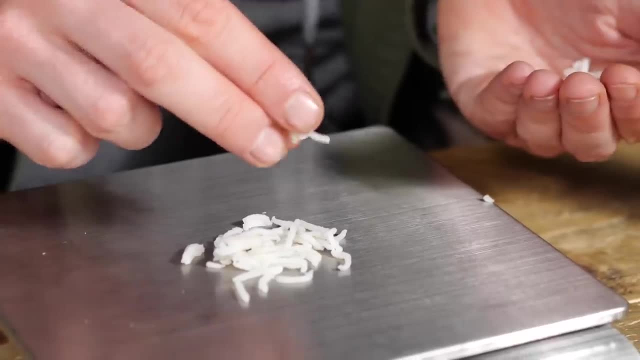 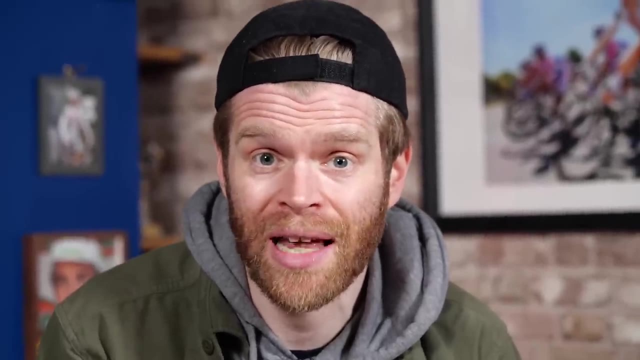 hanging out with friends and social occasions, because they become anxious at the fact that they're not going to be able to control this element of their lives and the things that they're potentially going to be putting in their mouths. What are you doing? Then there's the impact of cooking. 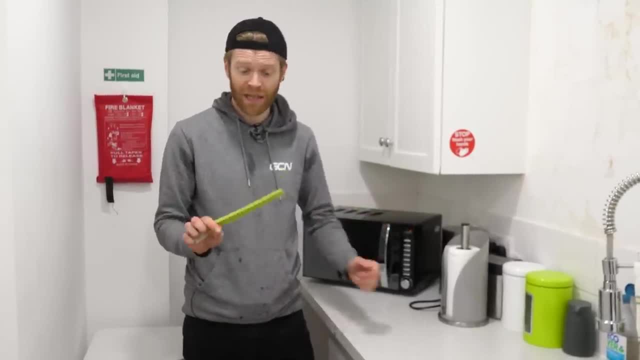 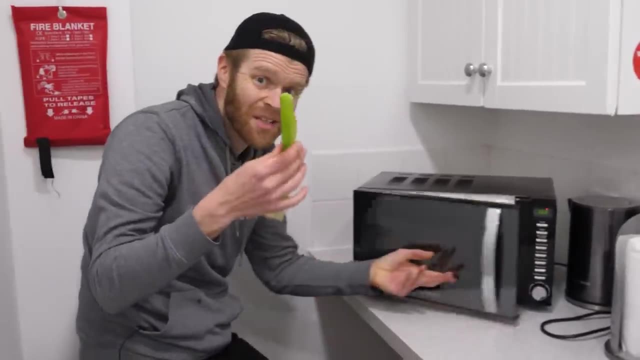 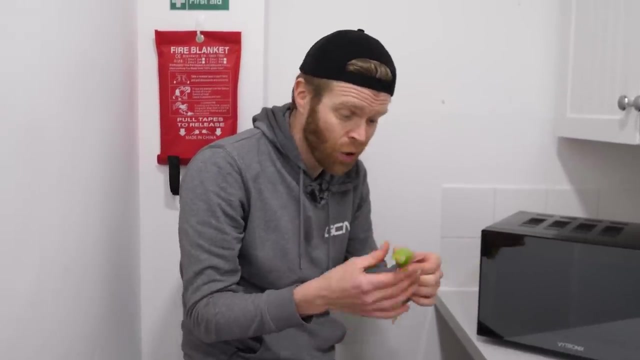 Food labels don't take this into account. A raw stick of celery has six calories, but once cooked it has six times that- 36 calories Across the board. cooking generally tends to alter the caloric content of food, meaning that it's very easy to miscalculate. 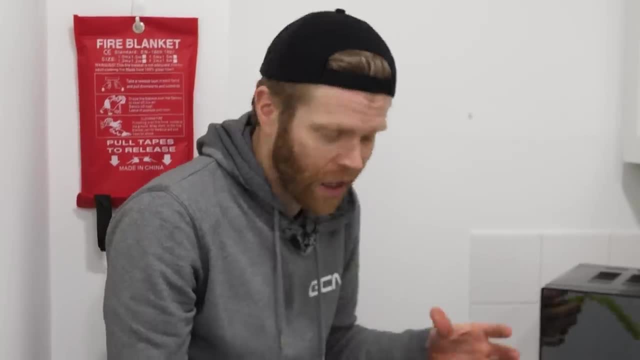 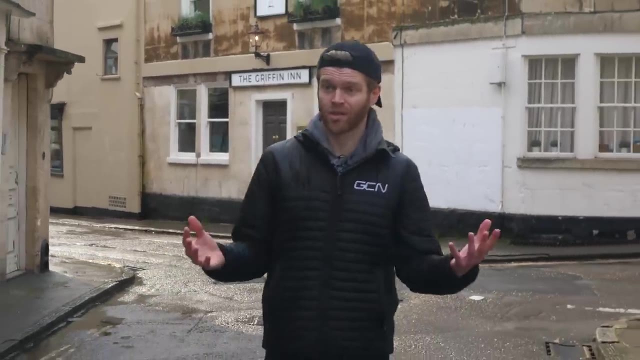 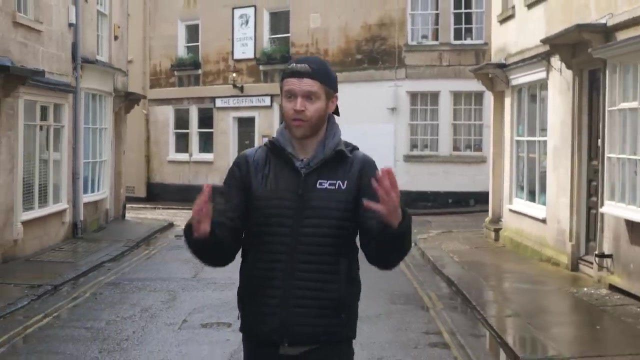 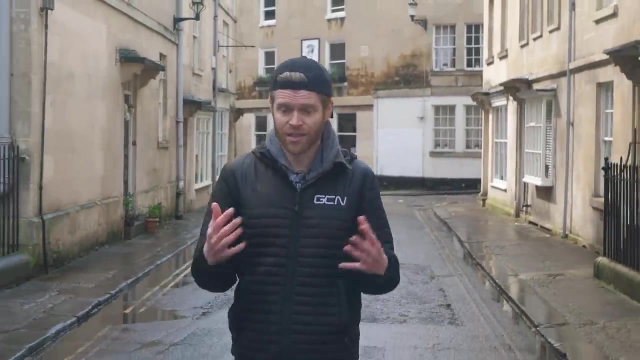 and overconsume. It's really hot, Disgusting. Reason three is the amount of calories that your body burns on a daily basis varies a lot and is also difficult to measure accurately. The go-to figures are 2,500 calories for men and 2,000 calories for women, While some calculators do account and adjust for your height. 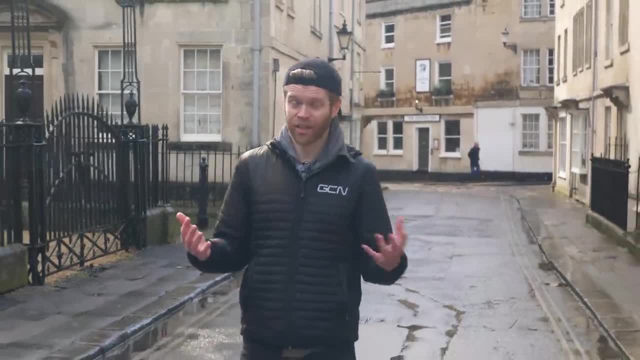 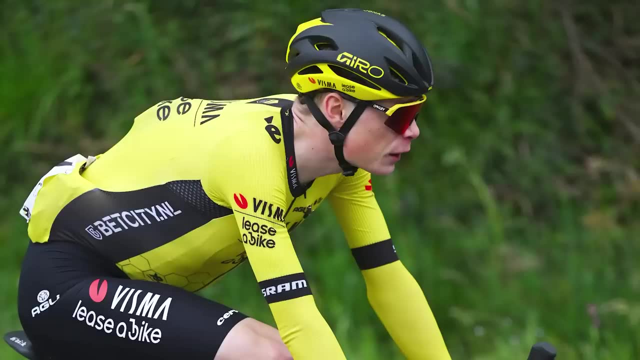 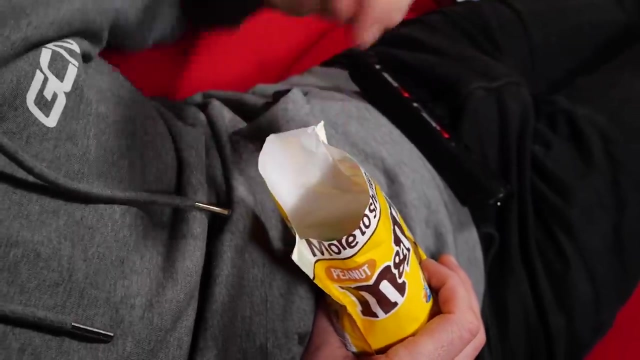 weight and age. this is still a gross oversimplification. 80-kilogram Filippo Ganna is going to burn significantly more calories than 58-kilogram Jonas Vingegaard. The amount you move has a huge impact and your basal metabolic rate varies from day to day. 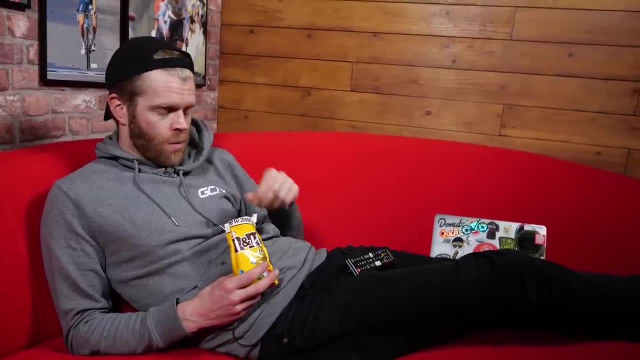 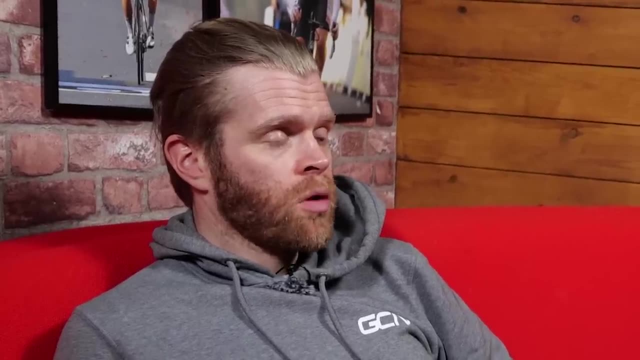 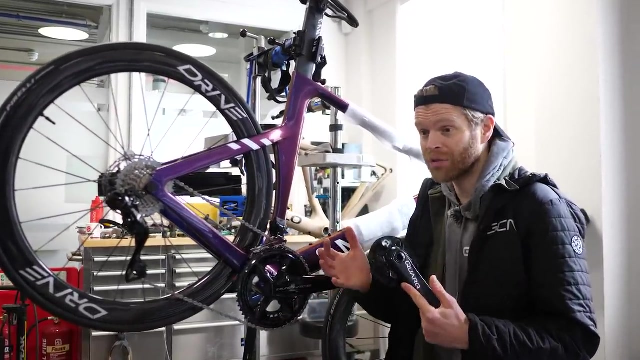 For example, if you're slightly ill and your body temperature is just 0.5 of a degree higher than normal, you're probably burning an extra 200 calories a day. Your power meter can accurately measure the amount of work done while riding, but it's not always clear how much of that was used. 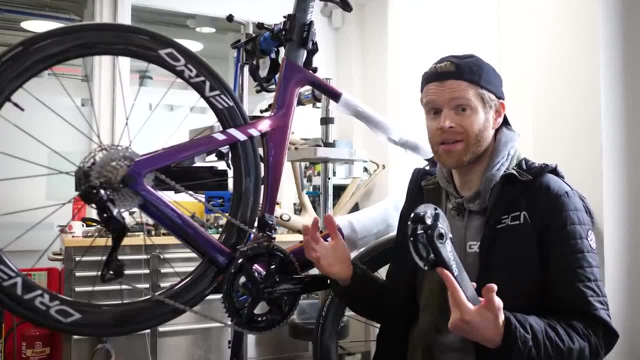 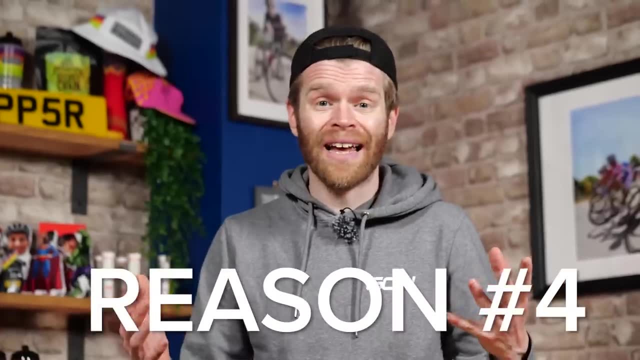 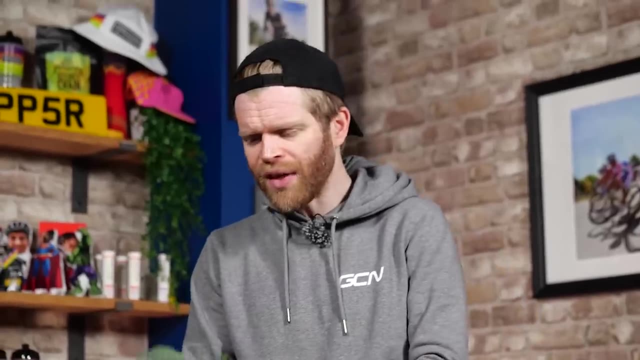 burning fat versus how much of that was used burning glycogen. Different power meters can also vary in their accuracy too. Reason four is that counting calories creates the perception that 1,000 calories of Mars bars is equal to 1,000 calories of broccoli. 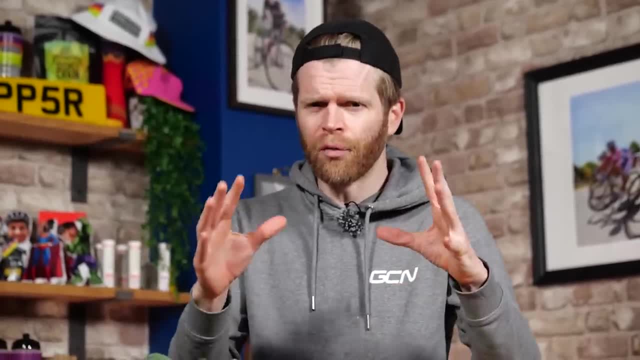 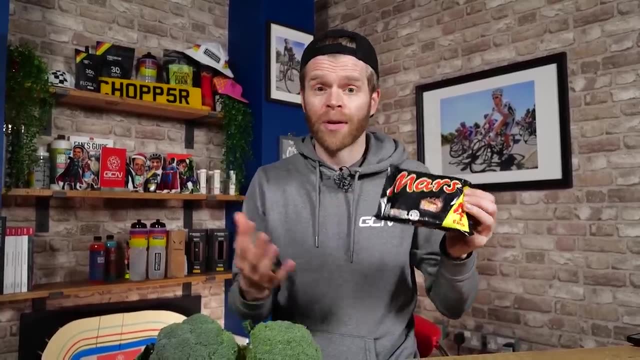 Now, big ultra-processed food corporations love people to think this, but it's clearly ridiculous. This contains next to no beneficial micronutrients, has had the fiber stripped out of it, contains loads of refined sugar and fat. This is an extreme example. 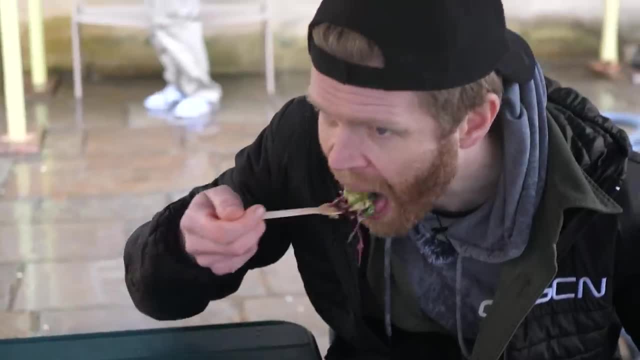 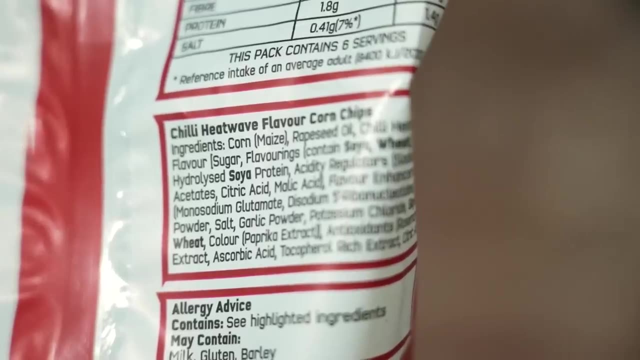 but you get the point. The reality is that it's much harder to overeat whole foods, whereas ultra-processed foods tend to be much more readily absorbed and also, when you eat them, are more likely to spike your blood sugar. A large part of this is probably because they've had most of their. 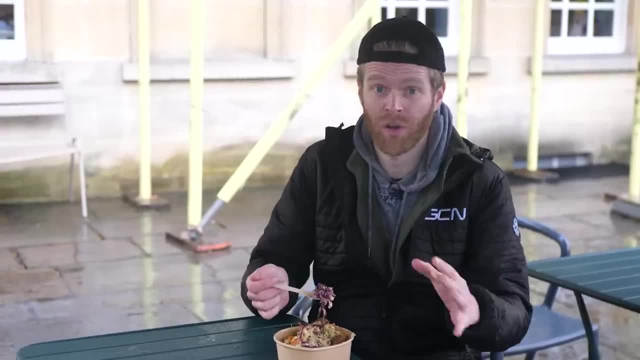 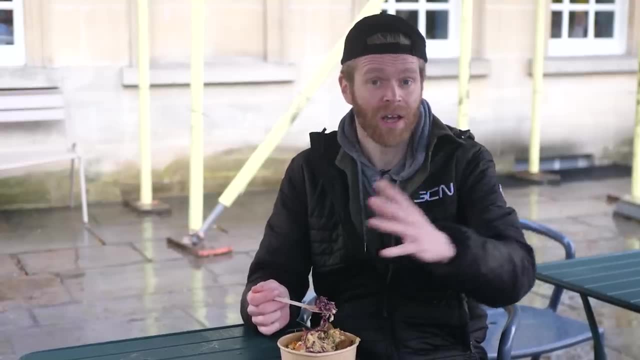 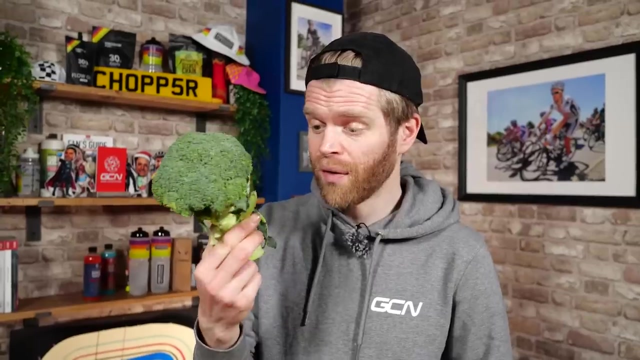 fiber content stripped out, and studies have shown that, when matched for macros, groups that eat a processed food versus groups of people that eat a diet of less processed whole foods tend to overconsume by 500 calories a day. Micronutrients and fiber just help you be more healthy. 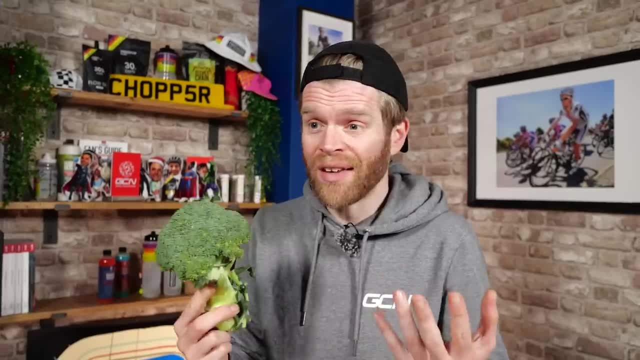 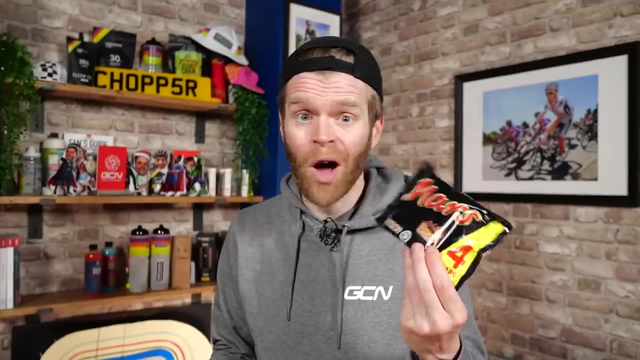 Irrespective of your weight goals. they're just something that you should consume in order to be healthier, whereas ultra-processed foods tend to be far more readily absorbed into the body and don't contain that stuff. You should also pay attention to macronutrients. Because they matter too. There is something to be said for the thermic effect of food, and something that's high in fiber or high in protein requires more energy to break down than just a refined carbohydrate. Calorie counting is a complete waste of time, Or is it Well? no, actually. 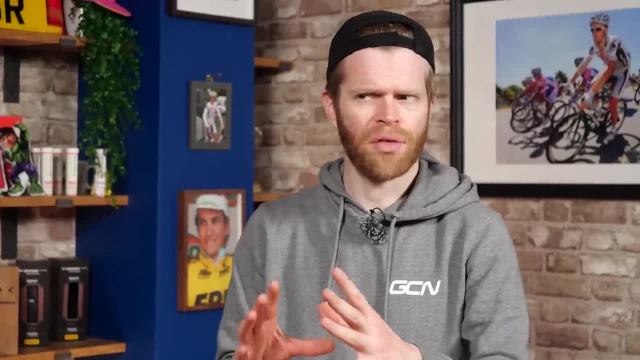 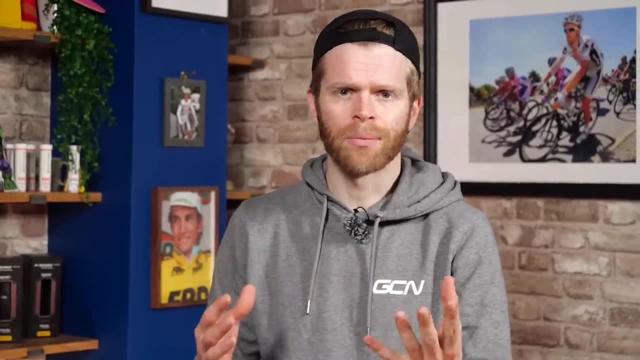 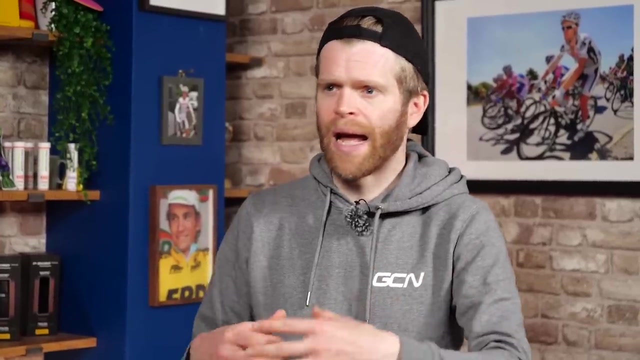 It's not a complete waste of time. The key thing to understand is that in theory, it's definitely possible that we could perform more accurate and precise measurements of energy in energy-out calculations. For example, 100 years ago we couldn't accurately measure the atomic. 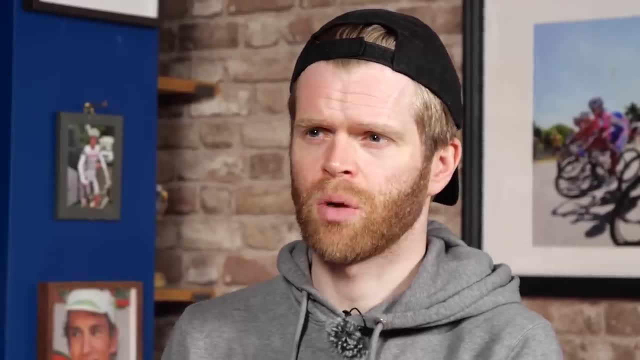 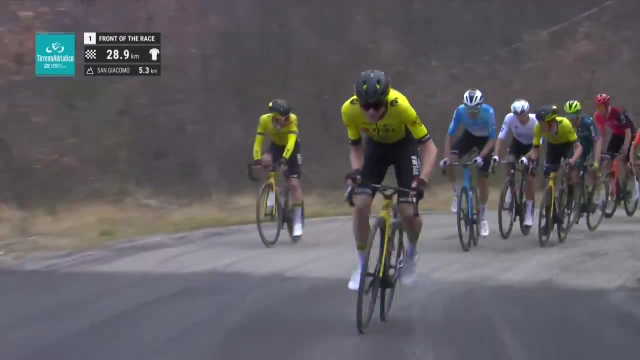 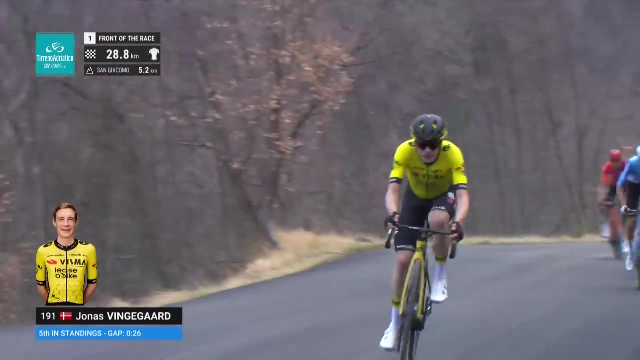 radius of a uranium atom, whereas now we canкой Vizmo Lease-A-Bike, the most successful cycling team in the world right now, are a team whose success is largely down to how lean their riders can be. They've used calorie counting to improve. 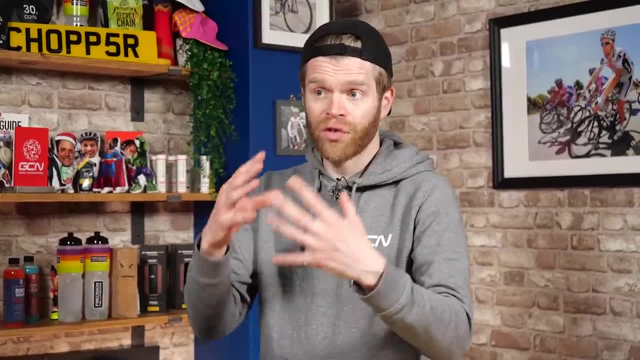 the riders' body composition, Although what they're doing is a more sophisticated, healthy, more prepragnant cycle speed that engineers can plan to perform every week or kick-off the holiday, Although what they're doing is steering doctors out of controlletter. las vaurs qq vessels, One of the�� 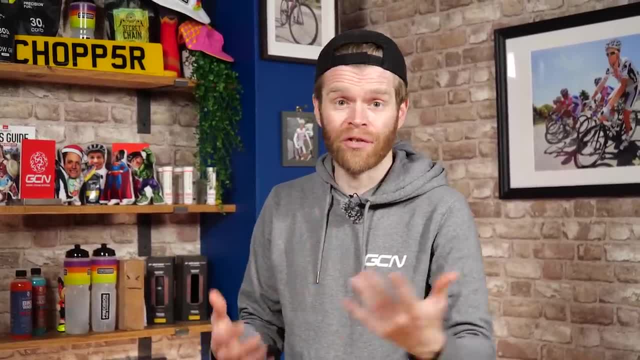 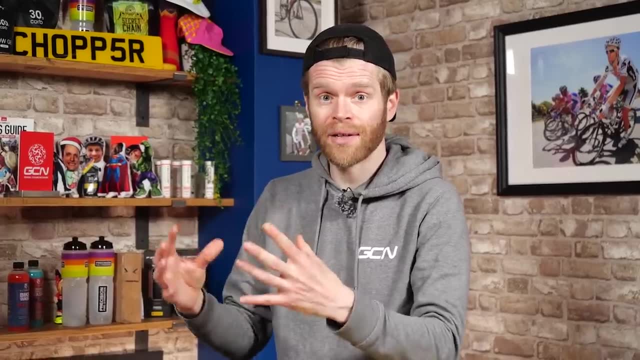 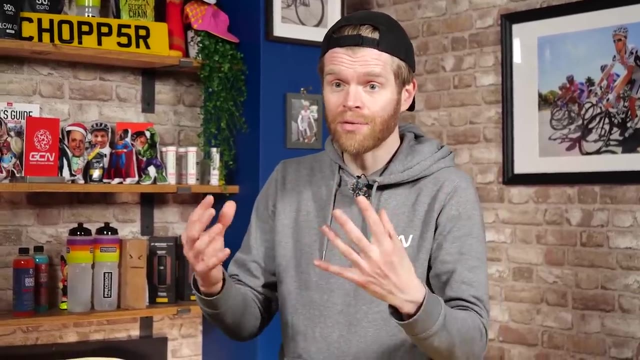 version of calorie counting that actually employs the use of a machine learning algorithm that can far more accurately predict the caloric demands of the riders for their training and racing. It actually is able to get more accurate over time the more they use it and the more data they give. 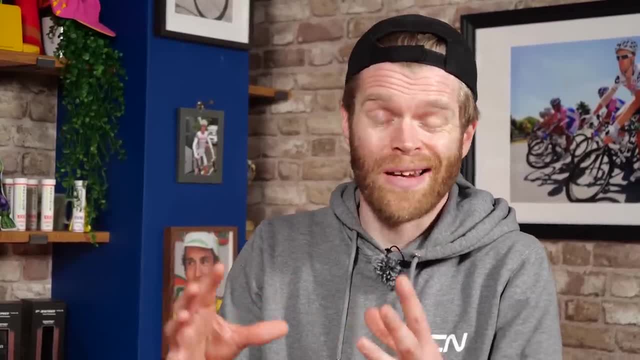 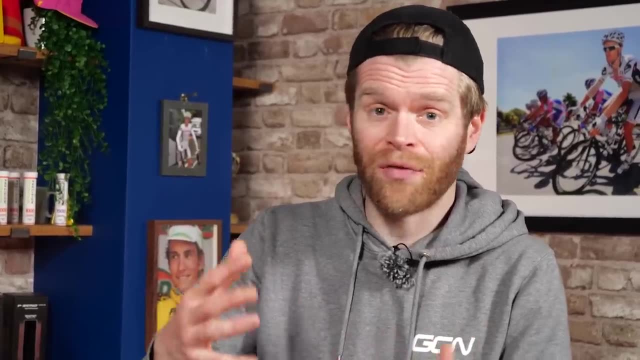 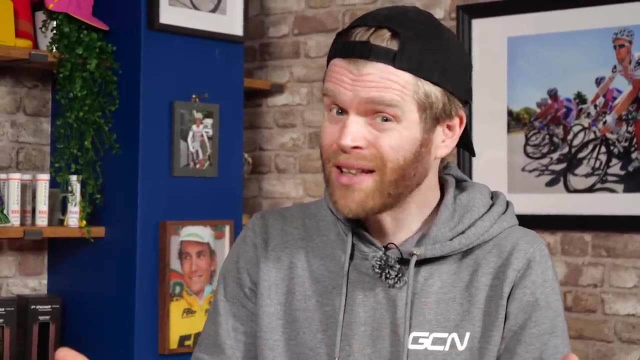 it. This isn't a mass market thing and it's nowhere near as sophisticated as what's theoretically possible, but it does show that, especially if things get even more accurate, that measuring energy in versus energy out in a more accurate way is a really useful tool. The other reason why it's 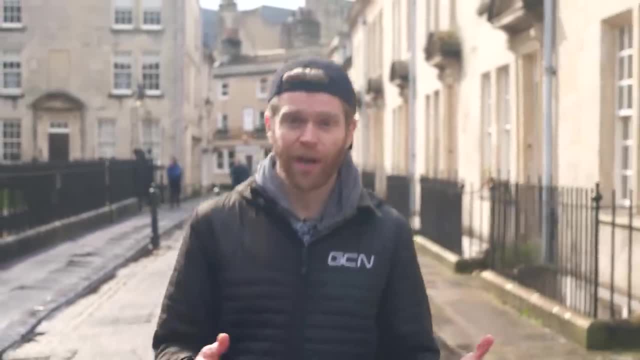 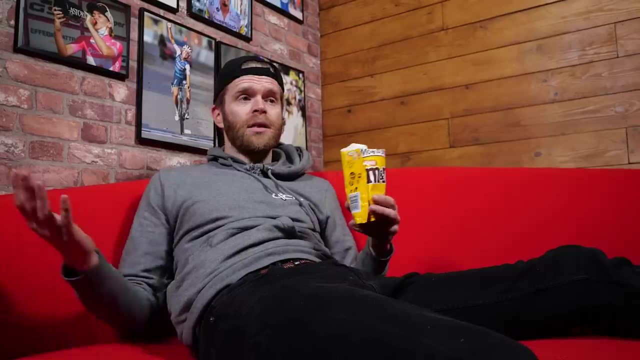 useful is through calorie counting, you're effectively keeping a food diary, and this is a really useful way of making you take notice of what you're actually eating and holding yourself accountable for it. This sounds obvious, but people often don't realize that they're snacking too much. 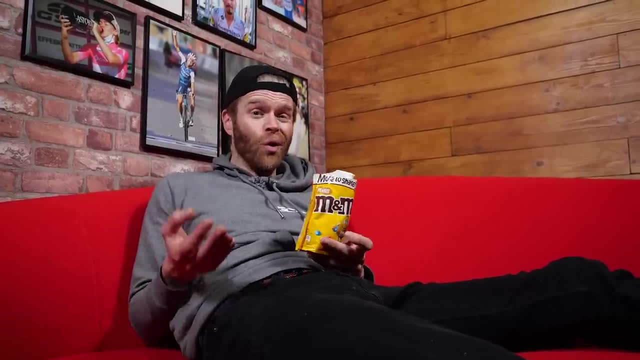 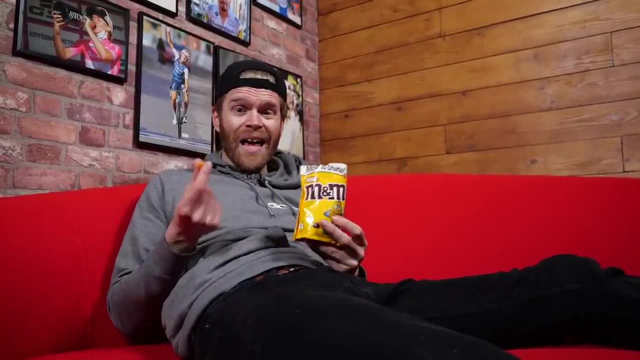 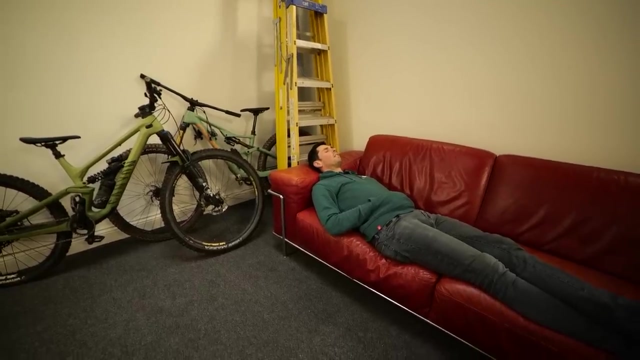 or eating too much much fat, Simply by keeping a record of what you're actually stuffing in your mouth. you'll probably be surprised at how the little things just add up. That full pack of Jaffa Cakes on the sofa after your training session probably isn't helping things. It can also be useful in 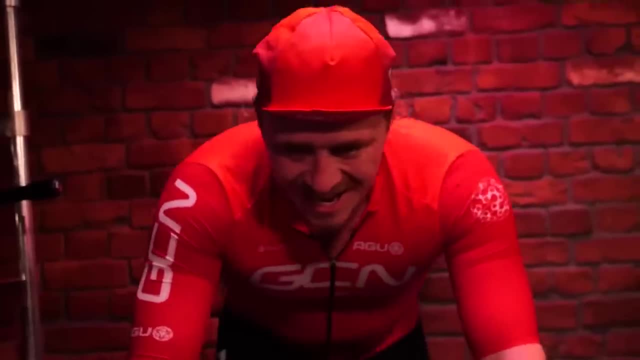 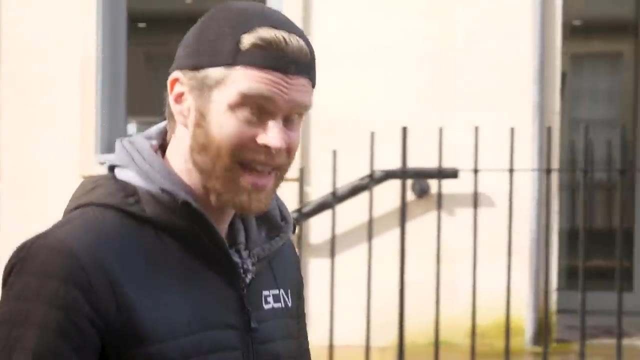 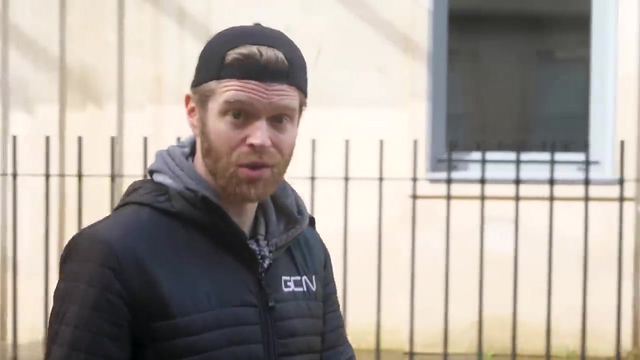 making sure you properly fuel your training sessions and get sufficient protein to recover. It sounds simple, but the single biggest thing that has helped me improve as a cyclist is making sure that I fuel properly and get enough carbs ahead of hard sessions or races or events. My 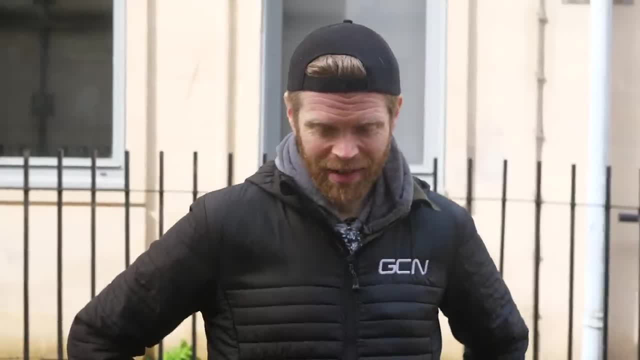 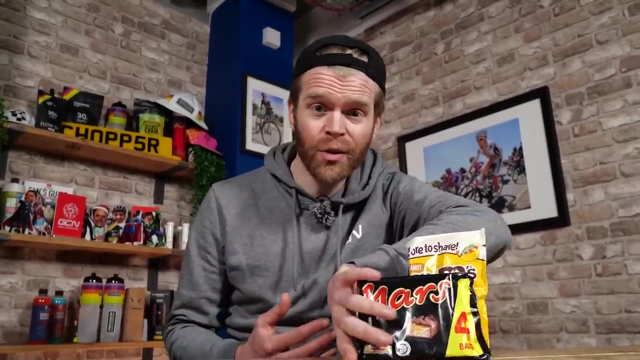 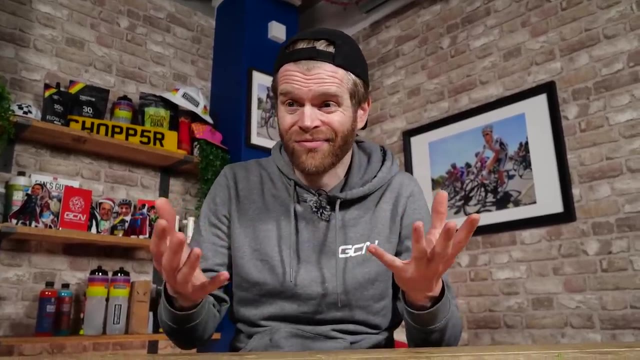 favorite things are pasta, porridge and rice. I love carbs. Now here's the thing: If you're limiting the amount of ultra-processed food that you eat and you're exercising a lot, you're getting fitter, but you're still putting on fat and getting fatter, then it's probably time that. 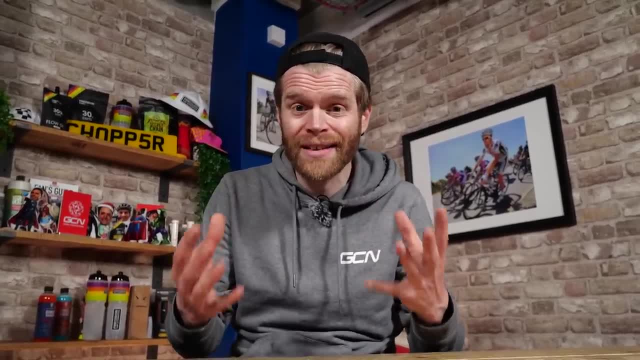 you actually make a note of the amount of carbs that you're eating and the amount of fat that you're eating. Make sure you make a note of the things that you're eating on a day-to-day basis and maybe just reducing it a bit. You can call this calorie counting. That's one of the freedoms. 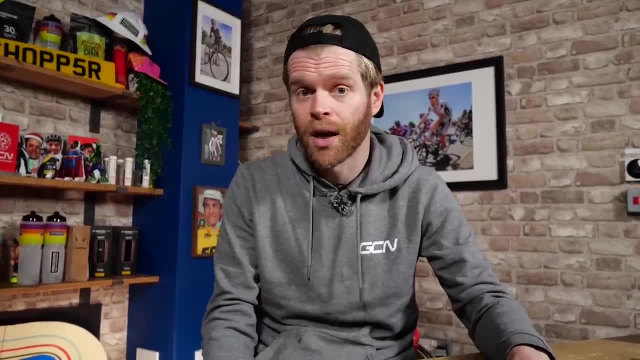 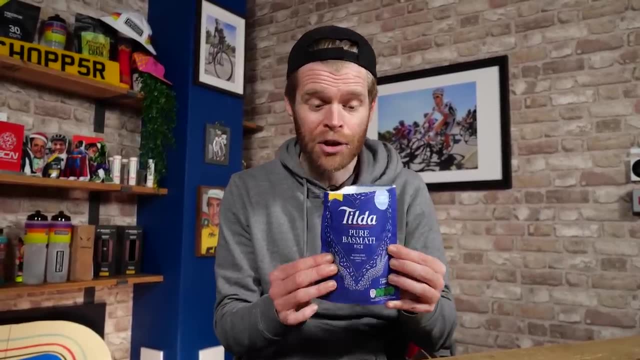 that's afforded to you, although I prefer to call it keeping a food diary. Now, another useful thing to do is to periodize your carbohydrate intake Ahead of hard training days and sessions. make sure you fuel for them and consume more carbohydrates compared to lighter days, where